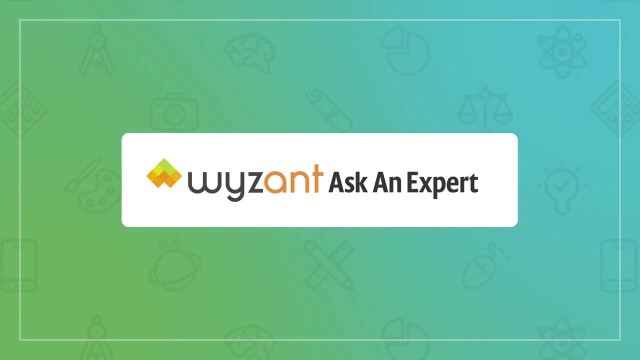 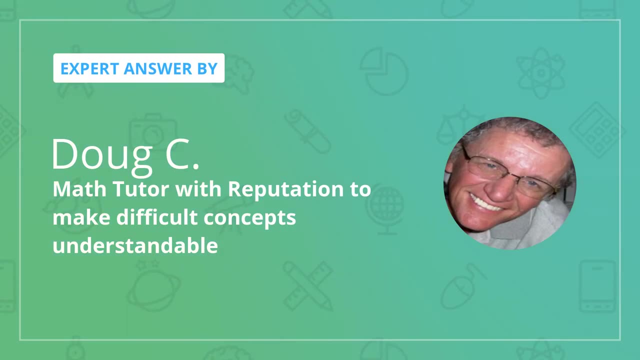 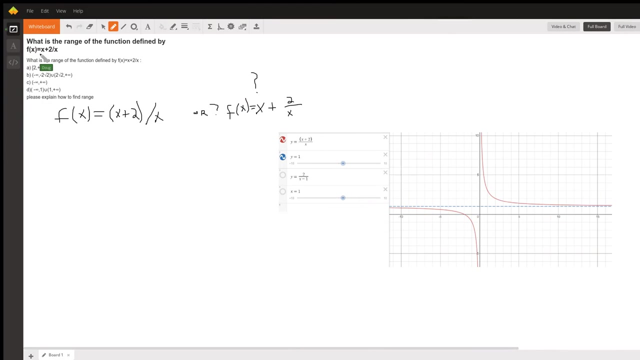 I'm going to hear about how this question is posed. If you're going to use this slash symbol, which is typical for asking a question about a defined function- and this is what you intend- then you should put parentheses around the x plus 2.. 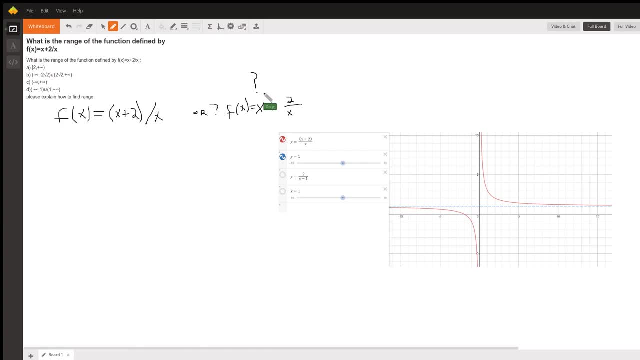 Otherwise somebody could interpret your question to mean this: Okay, that said, I've graphed the function over here on Desmos and it looks to me like the graph doesn't cross the line. y equals 1. And so this is probably the answer right here. 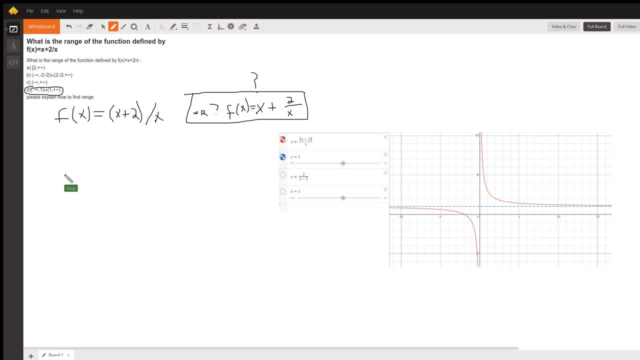 But is there a way to find that out without looking at a graph? Well, one way to do it is to realize that the domain or the range of this function is the domain. So find the inch of f of x. We might be able to. 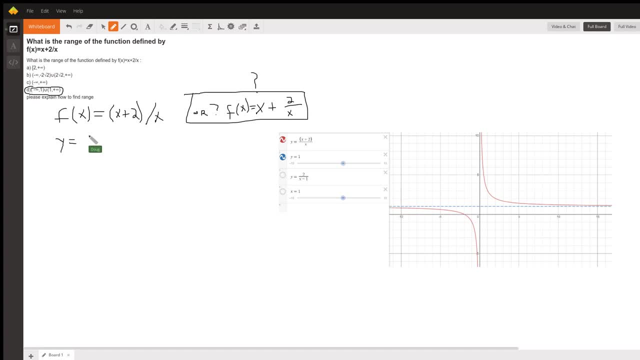 look at the domain and the inverse function and say, hey, I can't ever get this answer. So how do we find the inverse function? Well, the standard technique is to interchange x and y And then solve for y. By the way, we make note that x equals 0. 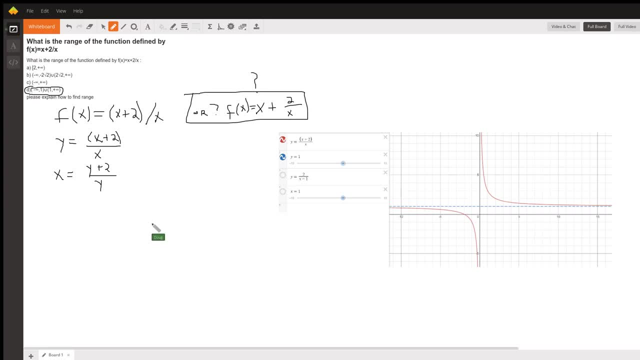 is not in the, in the domain of f, Because you can't divide by 0.. But if I want to solve both sides, or solve this equation for y, I might do something like this: Multiply both sides by y, Subtract y from both sides. 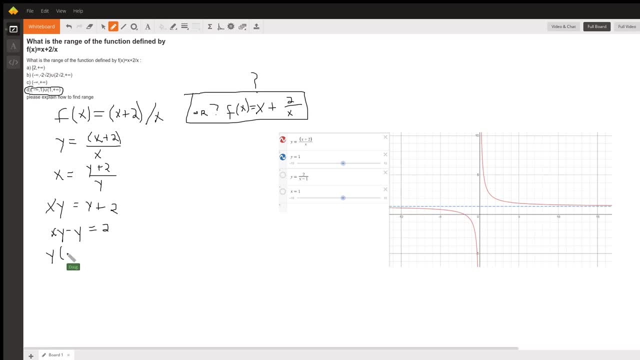 Factor out the y And then divide both sides by quantity x minus 1.. Now I'm going to define this as x minus 1. And then divide both sides by quantity x minus 1.. And then divide both sides by quantity x minus 1.. 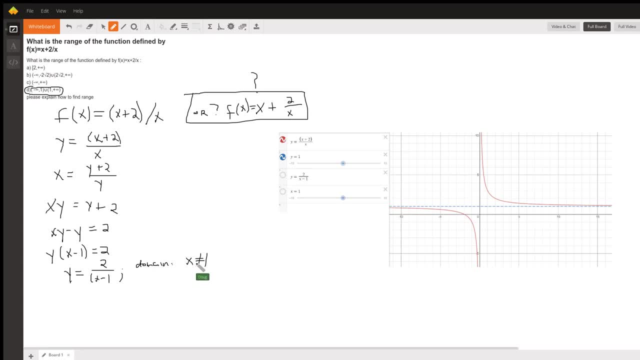 So the domain of the inverse function is all real numbers except x equals 1.. And that will be the range of the original function. And you might ask yourself this question: Will x plus 2 over x, will that ever equal 1?? 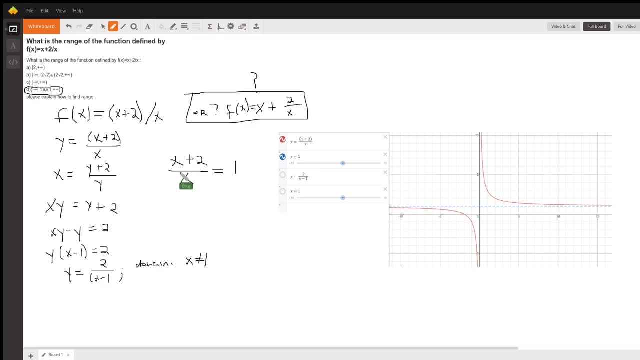 Just to convince yourself, Is there any number you could put in here for x that will generate an answer of 1?? And if you try to solve this for x, you get x plus 2 equals x, 2 equals 0. Therefore, solution set is the empty set. 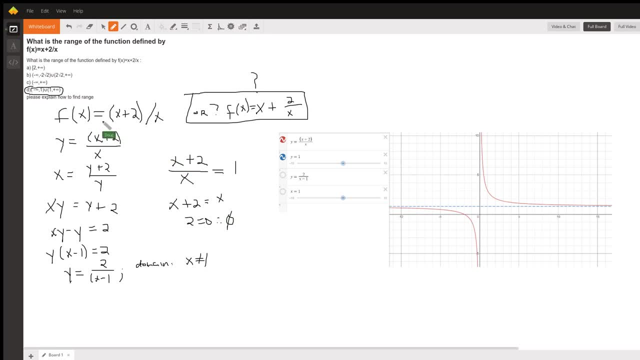 So there's no number x that you can plug in here. that will generate an answer of 1.. And that's why the range of this function is Using interval notation, from negative infinity to 1.. Joined with the open interval from 1 to positive infinity. There you go. 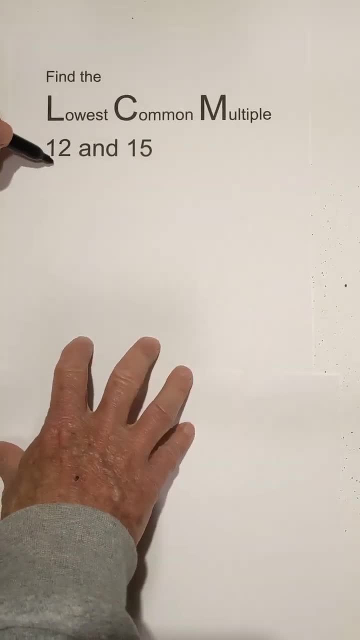 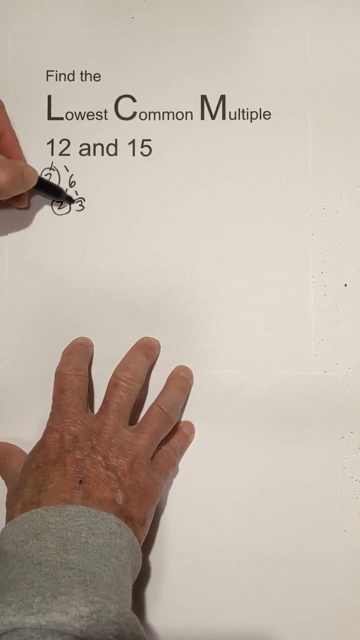 How do you find the lowest common multiple of 12 and 15?? I like to create a factor tree. 2 times 6 is 12.. 2 times 3 is 6.. I've circled the prime numbers 3 times 5.. They're both prime And then. 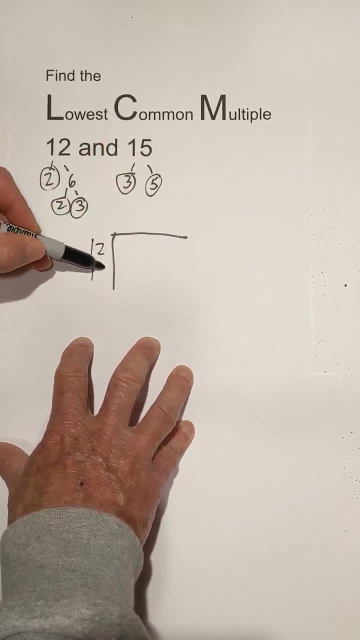 I put them in this nice chart. We've got 12.. We've got 15.. 12. I'm going 2, 2, 3. 15. I'm going 3 and 5.. The rule for the lowest common multiple: bring down the numbers If you have more than one.